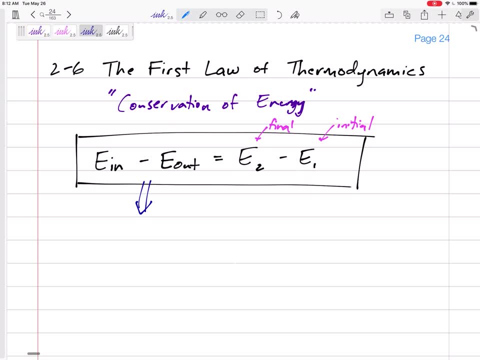 energy going in or out of our system, energy crossing the boundary right, Whereas the right-hand side of our system is the change in energy. So let's think about the left-hand side first and kind of say: you know, how can energy? 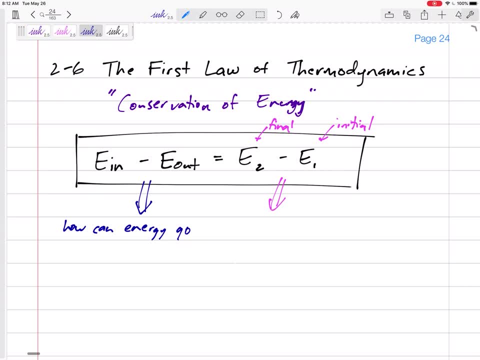 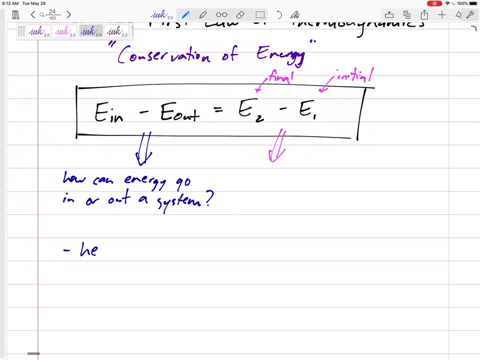 go into or out of a system. How can energy go into or out of a system? How can energy cross boundaries? Well, heat, Heat is a transfer, all right. Heat is an energy in or energy out. So we have energy out of our system Work. you know, do we have something adding work to our 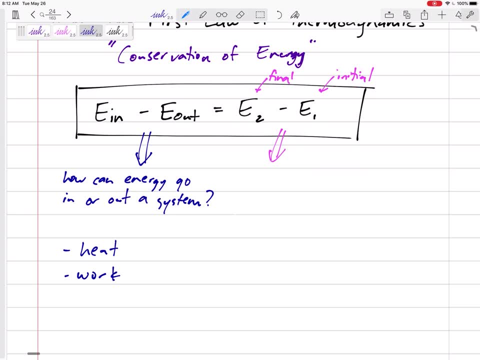 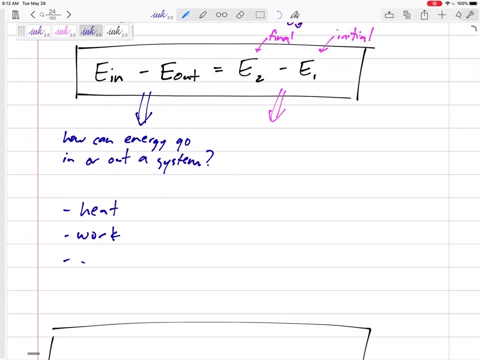 system. Do we have something taking work out of our system? Work is the left-hand side of our equation. And then also, if we just have fluid going into or out of our system, then the energy in the mass that is flowing in or out. 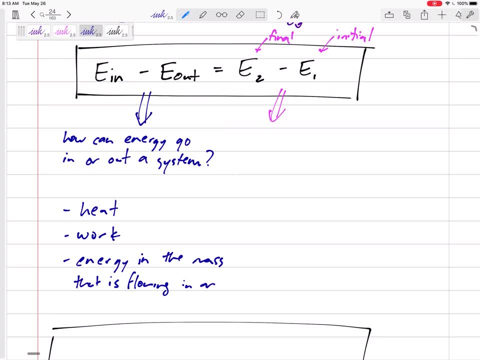 would be over here on the left-hand side of our equation. okay, So left-hand side, is energy going in or out, work being put into or work we get out of our system- heat transfer, or like inlet and outlet fluid. The right-hand side of our equation: let's think about what forms of energy. 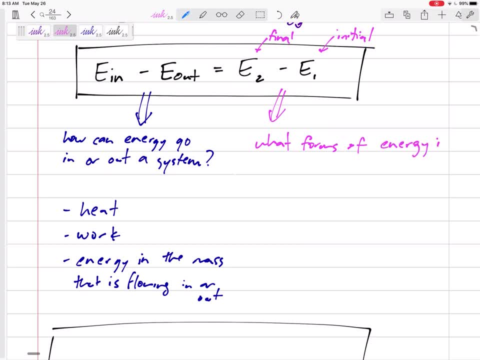 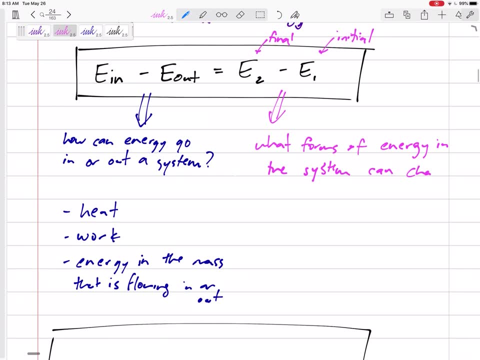 in the system can change. What forms can change? Well, maybe the kinetic energy. initially it's at one kinetic energy, one velocity, Final it's at a different velocity. Potential energy: potential energy: Right, maybe it's at one height, but afterwards it's at another height. 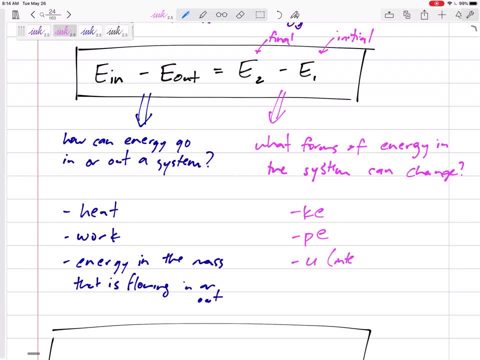 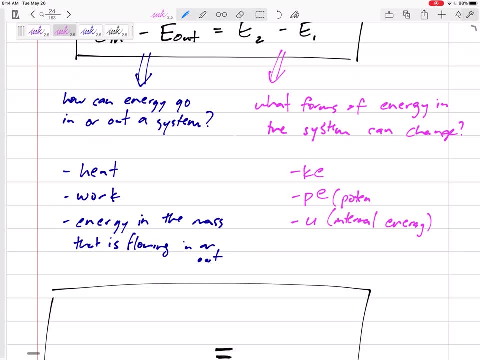 Internal energy. let me write these potential kinetic and maybe flow work. we'll tell you how we quantify flow work. Sometimes it's kind of on the right, sometimes it's on the left, sometimes it's combined with the flow going. 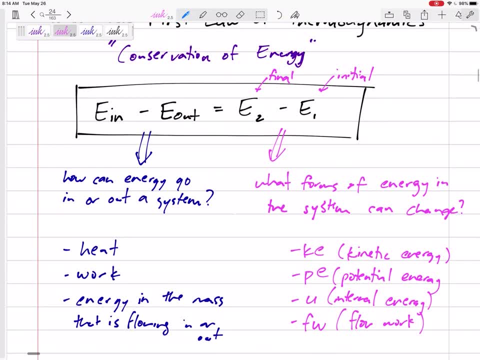 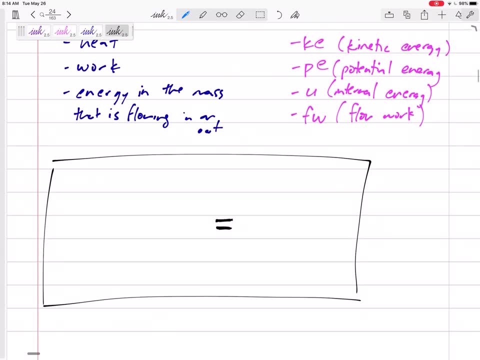 in and out. So there we go. So let's rewrite our conservation of energy equation with all these different types of energies So we might have heat transfer, maybe Q in or minus. if it's Q out We might have work. so we'll. 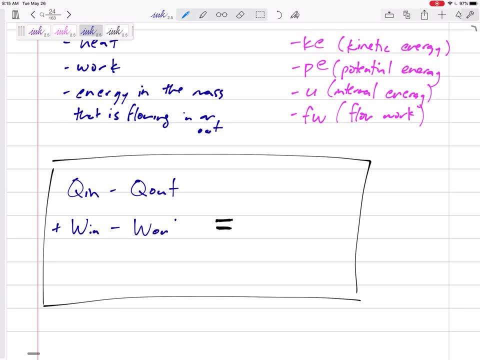 add work. if it's going in, we'll subtract work. if it's going out And we'll just say energy. if we've got energy in the fluid in, we add it, energy fluid out, we subtract it. And then on the right, 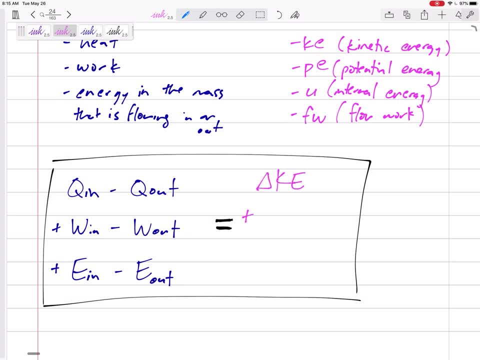 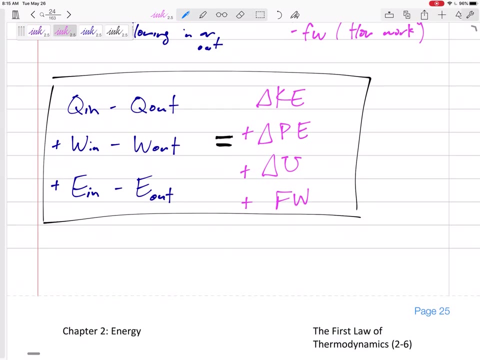 hand side. is there any change in kinetic energy? Is there any change in potential energy? Is there any change in internal energy And is there any flow? work right here. So there we go. That is our conservation of energy equation On the left hand. 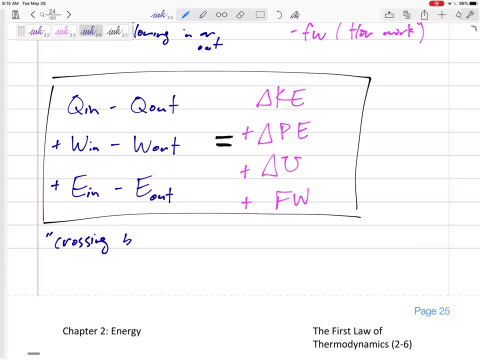 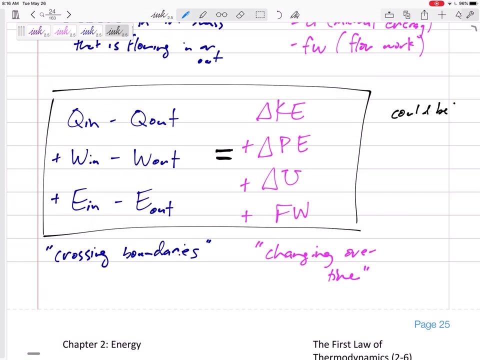 side, things that are kind of crossing boundaries, Whereas on the right hand side, things that are changing from beginning to end. Things that are changing from beginning to end. Now I put all these as capital. These could be capital E right like total, And you'll know that if the 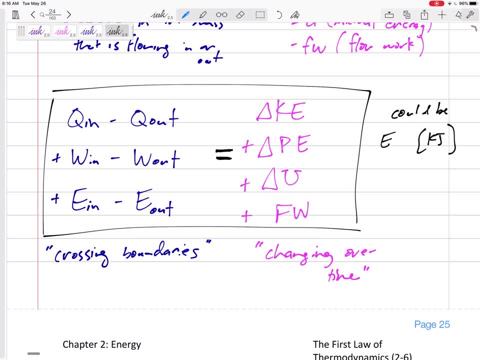 units are kilojoules or joules, All right, so this could be the total conservation of energy, But maybe all of this throughout. this whole equation is lowercase is specific. The unit is equal to the total conservation of energy, All right. 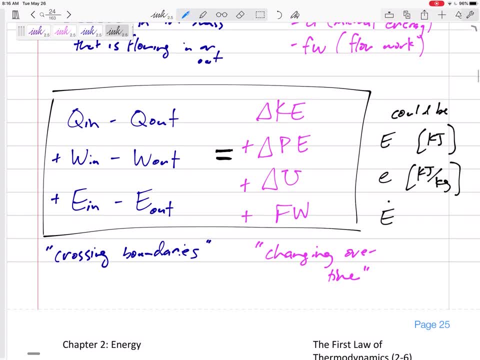 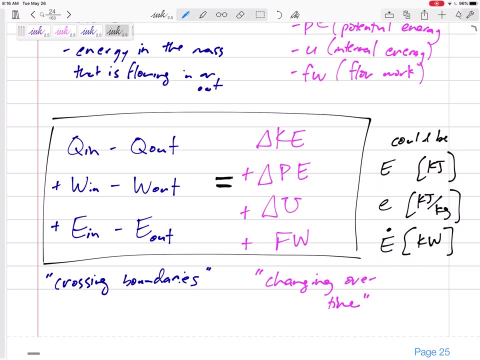 units would be like kilojoules per kilogram, Maybe it is all power, you know per time where it's units of kilowatts, And we have equations for all of these, most of these, for all three different scenarios, whether we're looking at total, specific.